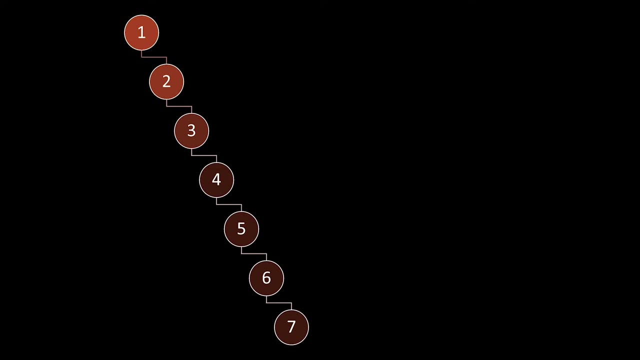 retrieving an item inside a list. So what AVL trees do to tackle this problem is make sure, every time we insert in or delete a node from the tree, that the tree is balanced. This is done by rotating or rearranging the nodes of the tree in a way that makes this: 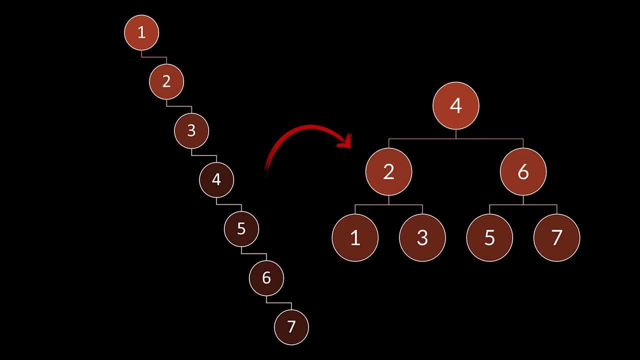 tree become balanced. Now, before diving in how exactly these nodes are being moved around, let's see when a tree or a node is balanced. Now, before diving in how exactly these nodes are being moved around, let's see when a tree or a node is balanced. 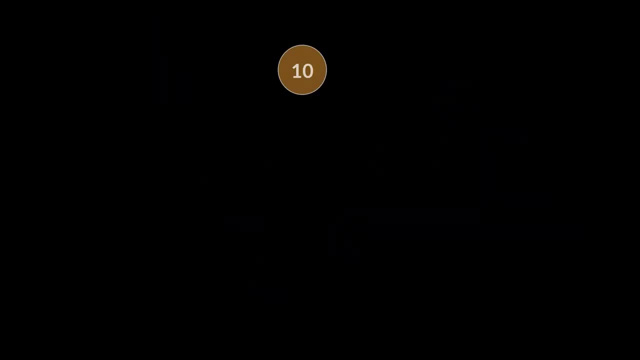 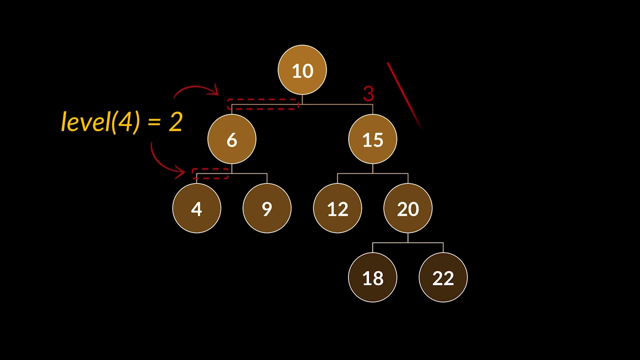 Now, before diving in how exactly these nodes are being moved around, let's see when a tree or a node is balanced. We previously discussed that the level of a node is the number of edges between the root node and the node in question, and that the height of a tree is the maximum level found. 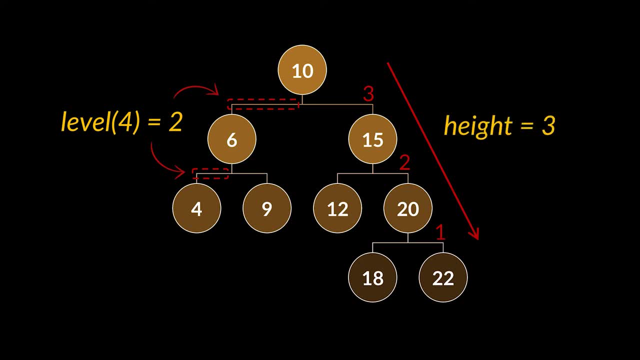 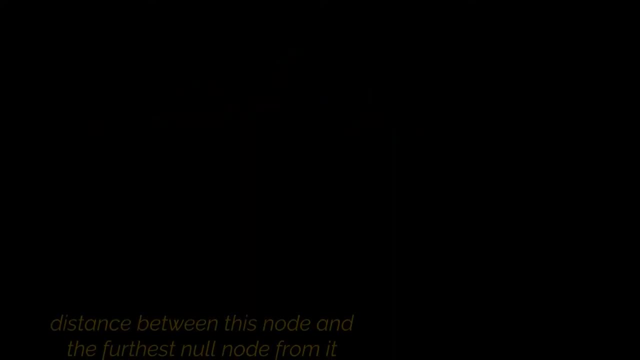 inside a tree, or in other words, the number of edges between the root node and the farthest node in the tree. Now, what about the height of a node? Similarly to the previous definition, the height of a node is the distance between this node and the furthest null node from it. Take this tree as an example. A leaf node has a single edge between itself and its null children, hence its height is 1.. A null node has obviously a height equal to 0, and the remaining nodes can now be easily guessed, as you can see in front of you. 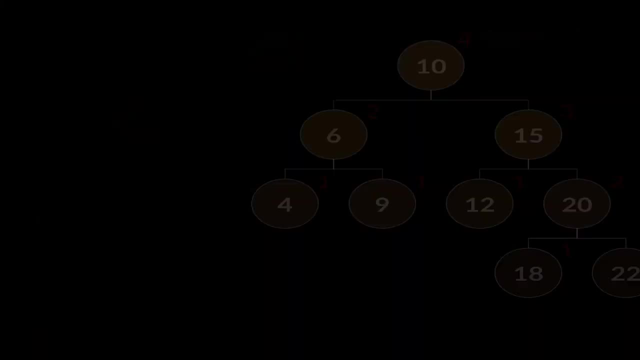 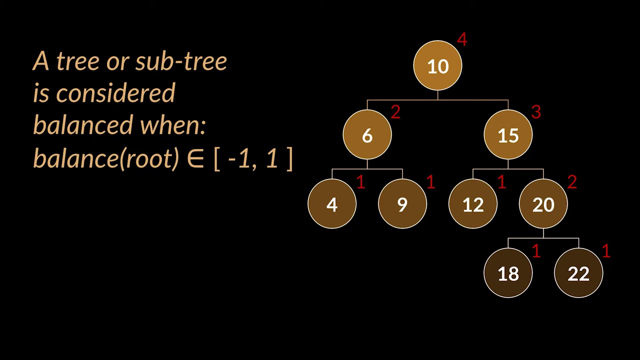 But why do we need this definition? Because a tree or subtree is considered balanced when the balance of its root node is smaller than 1, or bigger than minus 1.. And what is the balance of a node? Well, it is the difference between the heights of its left and right children. 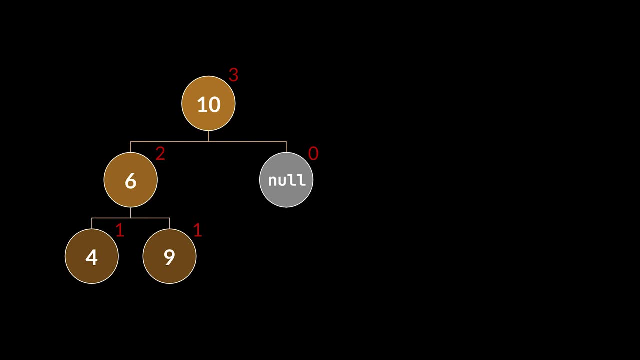 Take a look at node 10,, or the root node of this tree. The height of its left node, or left subtree's root, is 2,, whereas the height of its right node, which is the root of its right subtree, is 0,, as it is a null node. 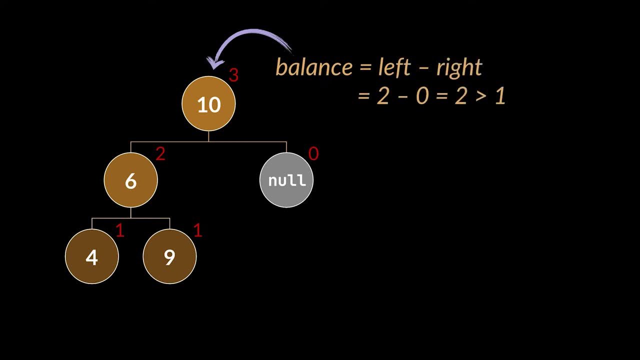 Therefore, the balance of the root node is 2 minus 0 equals 2.. Hence, these nodes need to be rearranged in a way to make this tree balanced. So how are we going to do that? The answer is rotations. 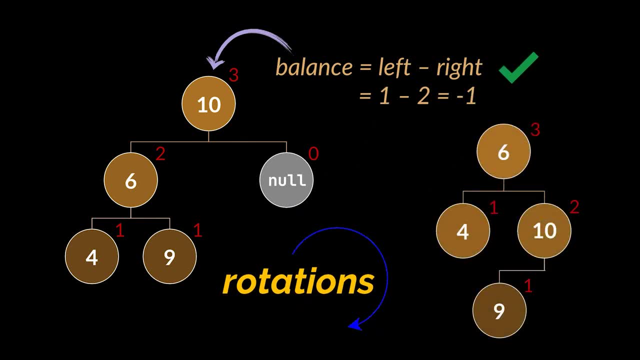 What a rotation will do is take the root node and rotate it to the right, as you can see in front of you. After doing this rotation, you can clearly see that the height of the left node of the new root is now equal to 1,. 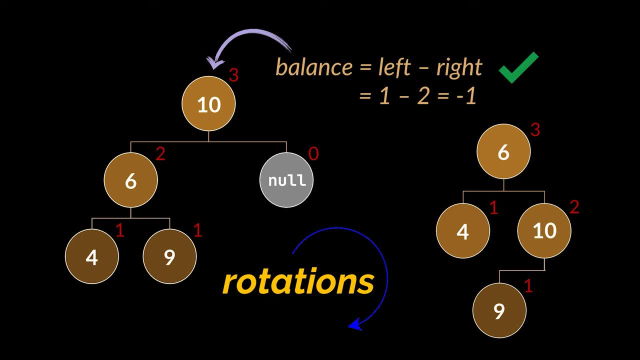 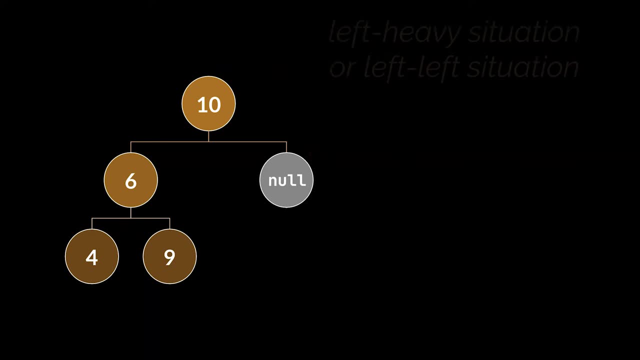 making the balance of the tree's root equal to 1 minus 2, equal minus 1.. Hence, this tree, with this one rotation, is now balanced. The case we just fixed using a single right rotation is what we call a left-heavy situation. 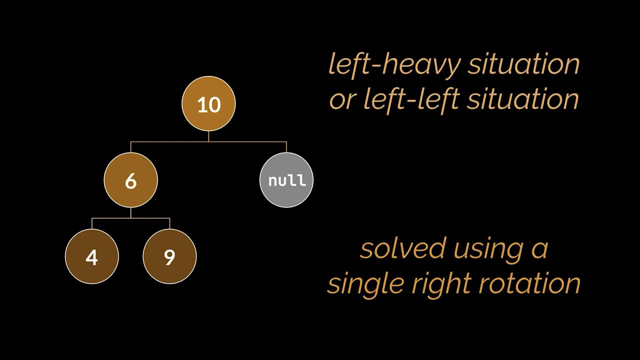 also referred to as a left-left-heavy situation. also referred to as a left-left-heavy situation. also referred to as a left-left-left-heavy situation. This case is encountered when the balance of a given node is greater than 1, as per our definition of balance. 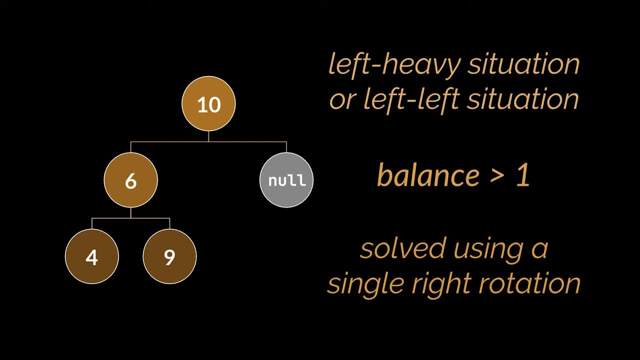 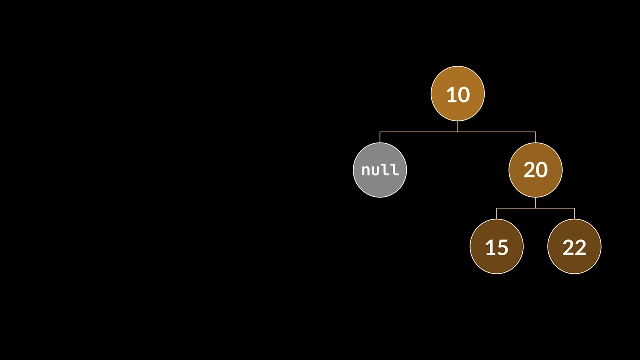 In addition to this scenario, there are three more cases we are going to discuss, making them in total four cases that should be checked every time we insert or remove an item from a tree in order to ensure and keep the tree balanced. The second case is very similar to the previous one, as it is symmetric to it in regard to the tree. 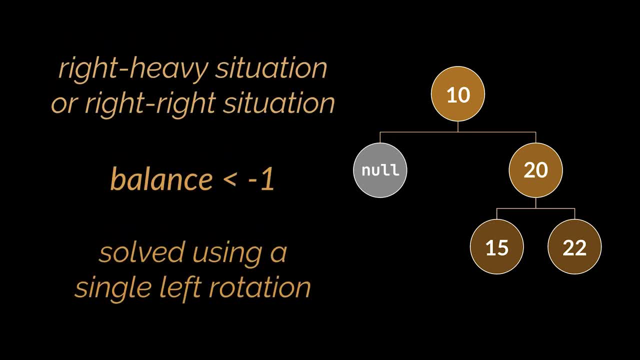 So, instead of having a left-heavy situation, we are going to have a right-heavy situation. So, instead of having a left-heavy situation, we are going to have a right-heavy situation. So, instead of having a left-heavy situation, we are going to have a right-heavy situation. 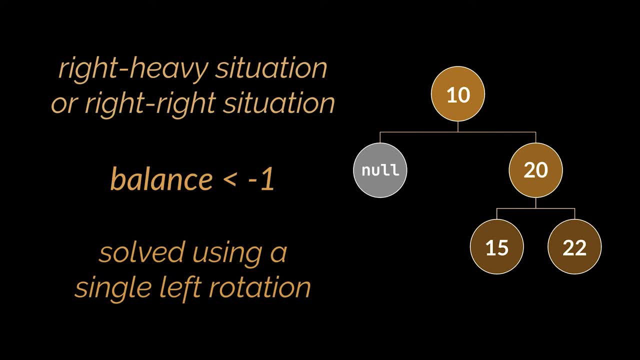 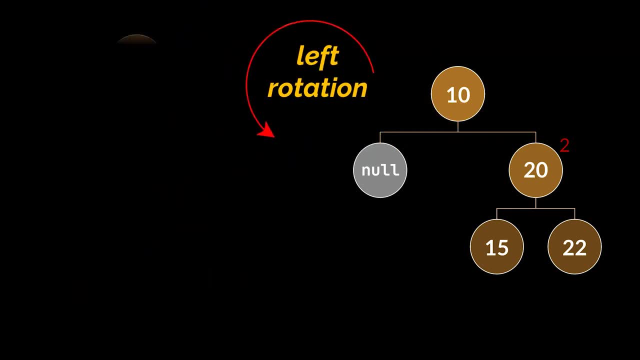 as the balance of the root node is now minus 2.. The solution to such an unbalanced tree is- you guessed it- a left rotation. Hence, the unbalanced tree you see to your right-hand side, after applying a left rotation, will become the balanced tree you see to your left-hand side. 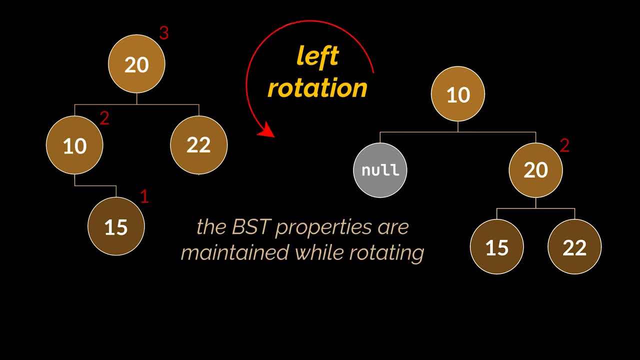 Notice that all the binary search tree properties are maintained while rotating and that the heights of the nodes we are rotating are being updated with every rotation. Now the third case may not be as straightforward as the previous one. Now, the third case may not be as straightforward as the previous one. 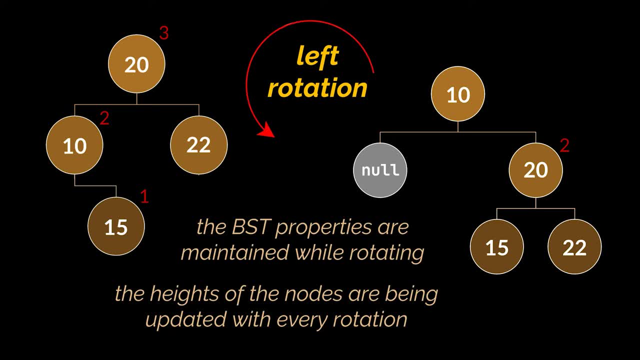 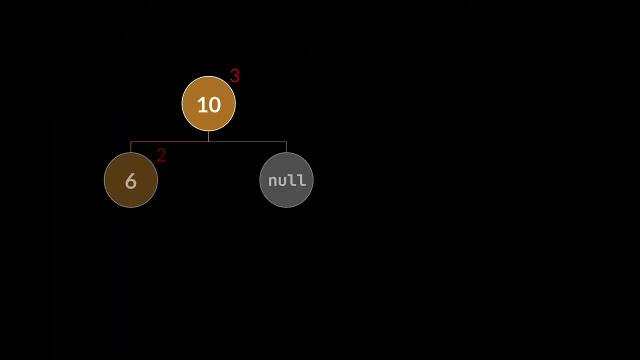 Now, the third case may not be as straightforward as the previous one, but once you get it, you will also get the last one, the fourth one, as they are symmetric, just like the first two cases were, The third case can be represented as such. 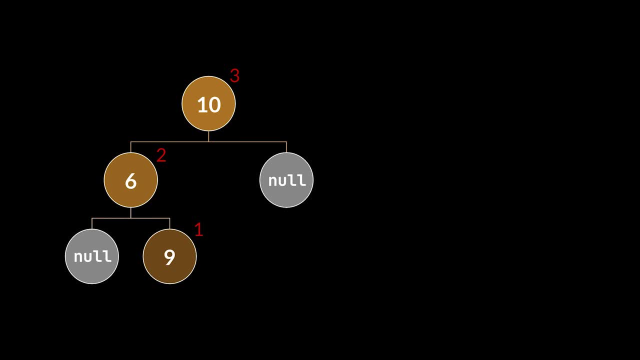 and from the heights of the nodes, you can see that the tree is unbalanced, as the balance of the root is equal to 2.. So, using rotations, we need to fix this tree, all while maintaining the binary search tree properties. 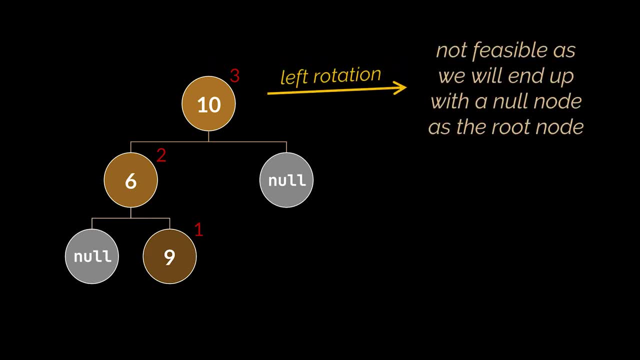 However, in this example, we can't do a left rotation because we will end up with a null node as the root node, and if we do a right rotation, we will end up with something like this. You see, this is even worse. 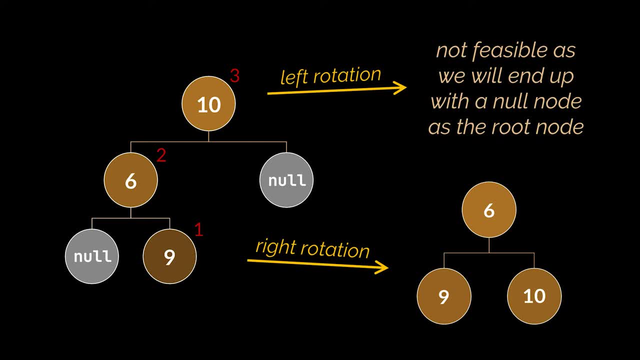 because the tree we obtained here violates the binary search tree properties. The left child we have here is now bigger than its parent, which is totally wrong. So how are we going to balance this tree? To do this, we have to start by performing a left rotation. 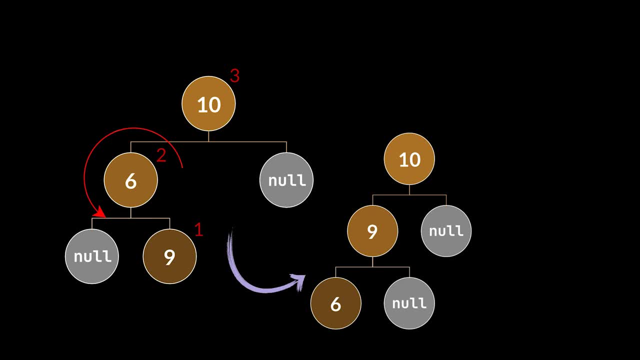 on the left child of the root node of the subtree we want to fix. By doing this, we will return right back to the left heavy situation, and now we already know how to fix this one using a right rotation. This scenario is referred to as a left-right situation. 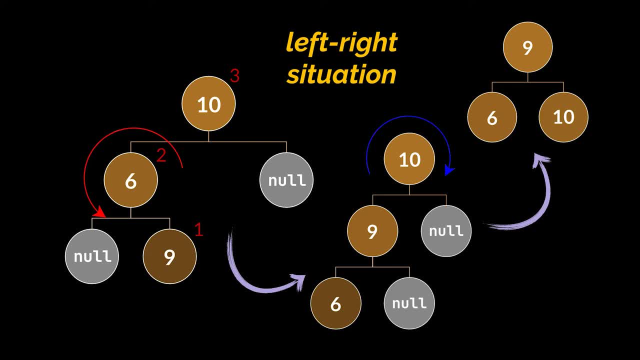 but how did we know that a left rotation is required here and on the left child in particular? You see, if we calculate the balance of the left child we rotated at first, we will obtain minus 1.. And always remember: negative balances mean left rotations. 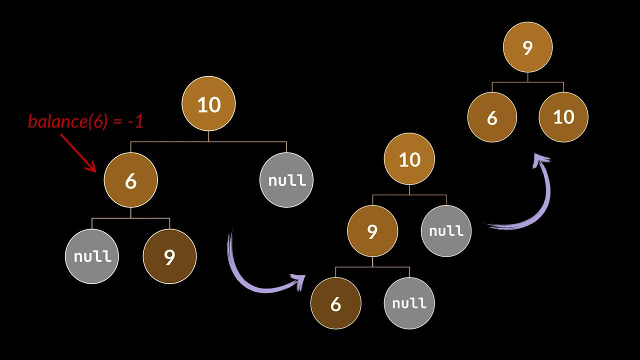 and positive balances mean right rotations. In a left heavy situation, this balance was equal to 1,, which means it has the same sign as its parent, but in a right situation the child is negative and the parent is positive, leading to a left rotation followed by a right rotation. 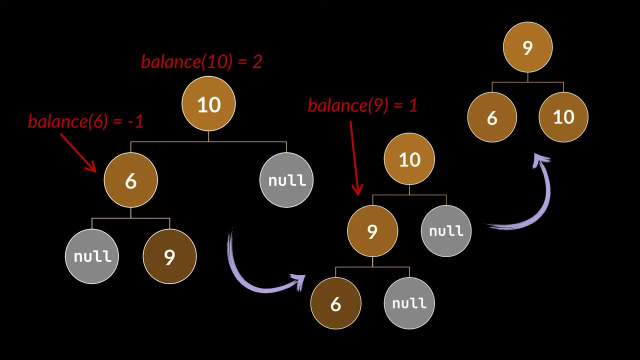 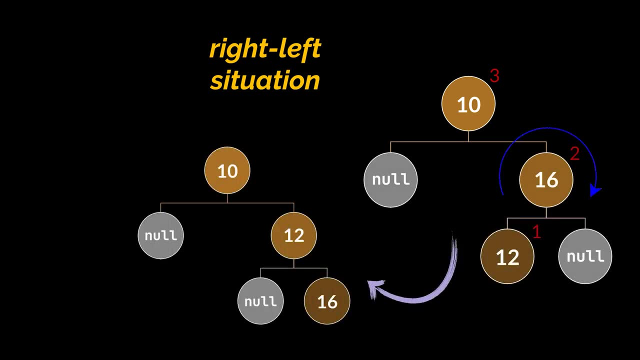 The fourth case should be pretty straightforward. now. I assume It is the right-left situation and it is symmetric to the third case we just covered. Here we need to apply a right rotation on the right child of the subtree's root. This rotation will place us in a position similar to the right heavy situation. 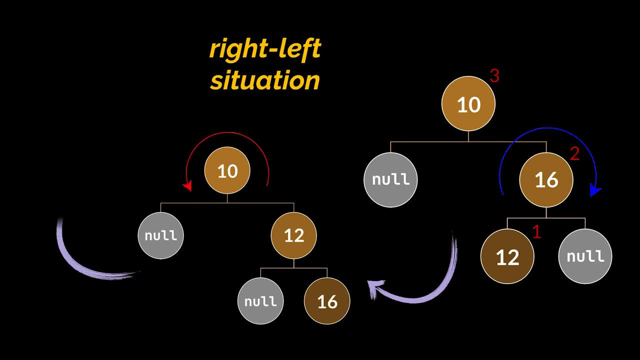 we already discussed. Now this can be solved using a left rotation on the root node of the tree itself. In this final situation we had that the root's balance was equal to minus 2, and the right child's balance was equal to 1.. 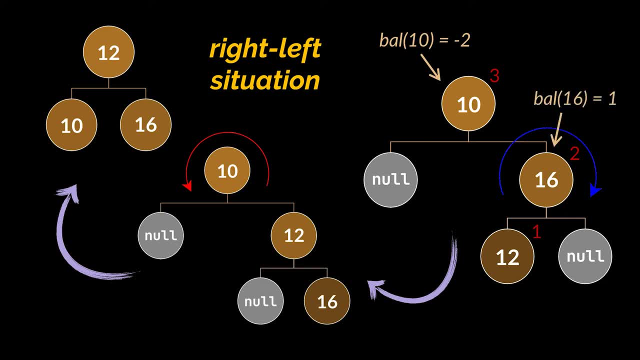 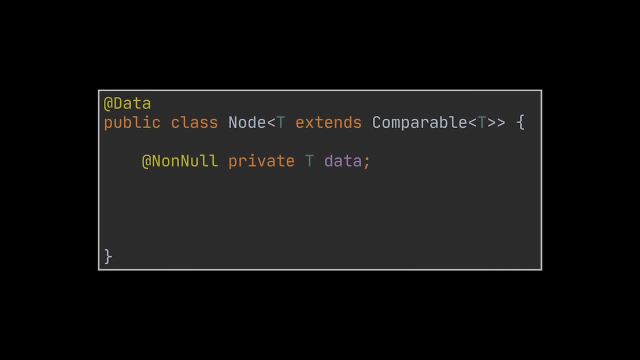 Okay. so, with all four unbalanced scenarios we covered, let's try to implement the AVL trees together, As we did for the binary search trees. we are going to start with the node class. This node will wrap our data and will hold its left and right children. 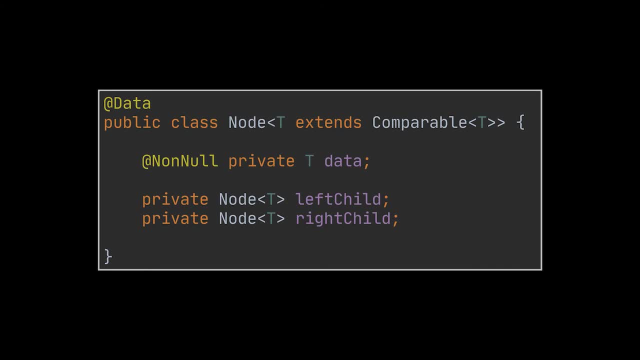 similarly to the binary search tree node. However, in addition to those, this class should keep track of the height of the node By default. this height upon which the tree is placed is the height of the node. The height upon creation of a new node is equal to 1,. 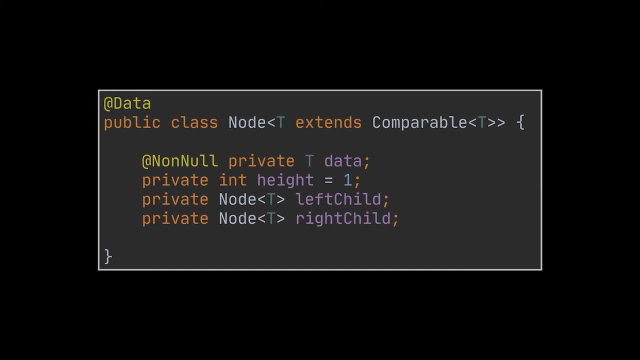 as when a node is created or inserted into an AVL tree, it is initially inserted a leaf node and the height of a leaf node is equal to 1.. Additionally, and same as we previously did, the data wrapped by the node is made generic. 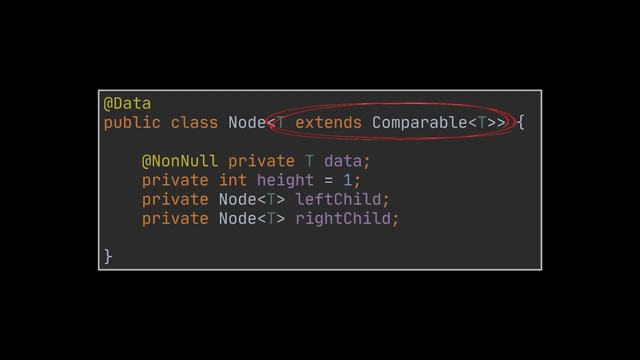 allowing us to hold and store any type of object we want. The annotations you see are Lombok annotations. Project Lombok is a dependency that provides several annotations which reduce boiler-place code, such as setters, getters, the two-string method, constructors and many more. 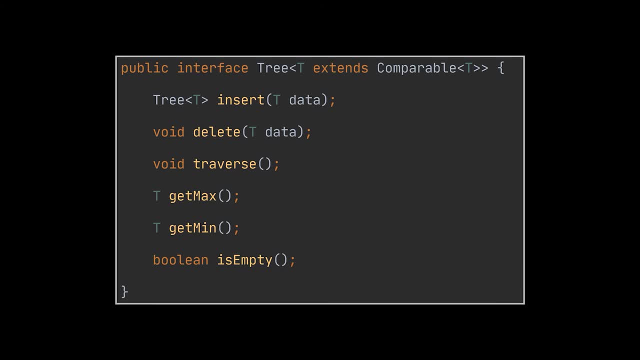 Now, before diving in AVL trees, take a look at the tree interface we will be implementing. Notice that it is exactly the same one we implemented in case of a binary search tree. And that is not all, because checking if the tree is empty or not. 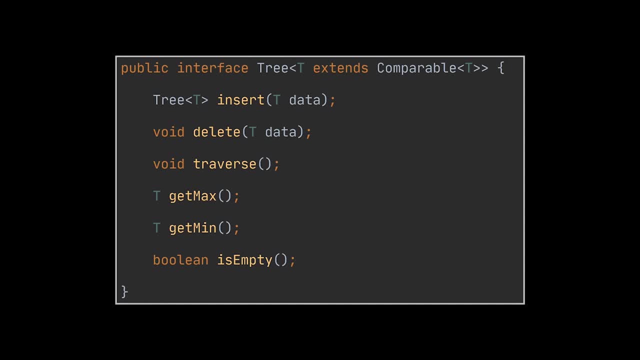 retrieving the maximum or minimum element from the tree and traversing a tree all have the exact same implementation to the one we did in the previous video of this series, the binary search tree video. So if you want to dive in the details of their implementations, 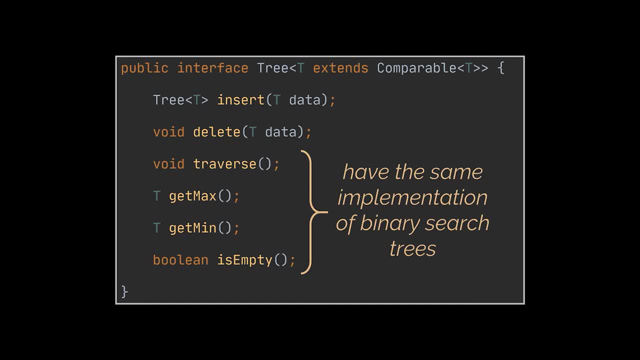 do take a look at the video linked in the description down below. What we are left with are the insert and delete operations. Both of these operations are actually also similar to the ones we implemented in our binary search tree video. However, what differs between the BST and the AVL tree? 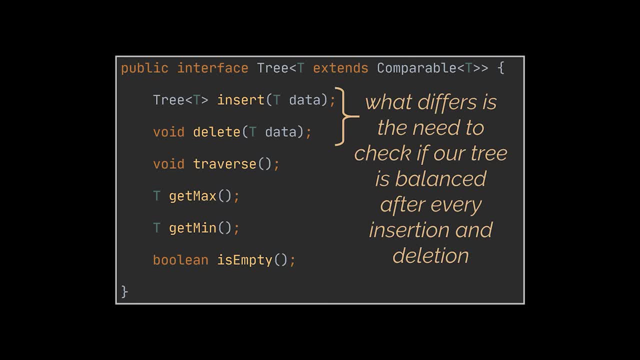 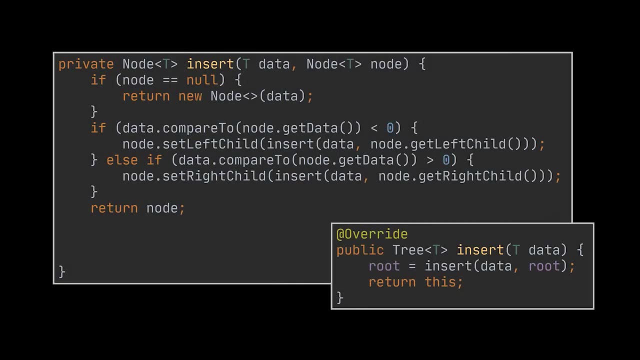 is that after every insertion and deletion we need to make sure that our tree is still balanced. So the insert method will look exactly the same as what we covered in that binary search tree video, but with a little twist. What you see is the implementation of that insert method for the binary search tree. 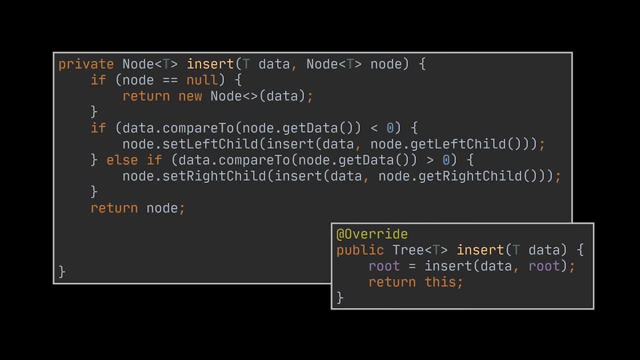 exactly as in the last video, but what we are going to do is add at the end of it, after our recursive calls, two checks. One of them will apply the needed rotations based on the four scenarios we discussed earlier, and the second one will update the height of the rotated node accordingly. 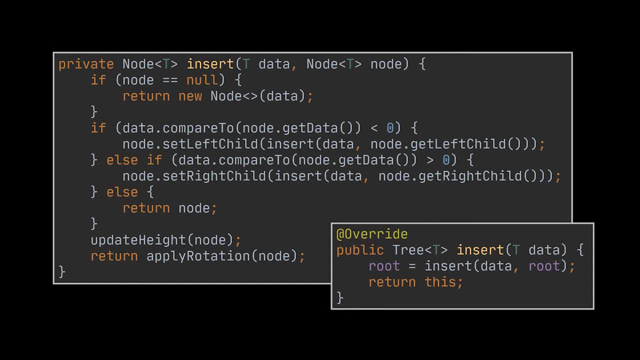 as rotating the nodes of our tree will most probably change their height. Don't worry, we are going to implement these two calls in a few, but not before mentioning that the same two calls should also be added at the end of the delete operation. 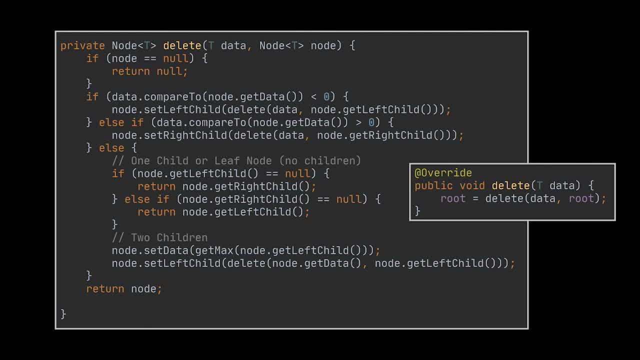 So what you can see here is the delete operation as we implemented it in the BST video, and to make it an AVL tree implementation, all we have to do is invoke these two methods right after we are done with the actual deletion. They will ensure that the height of our nodes is always up to date. 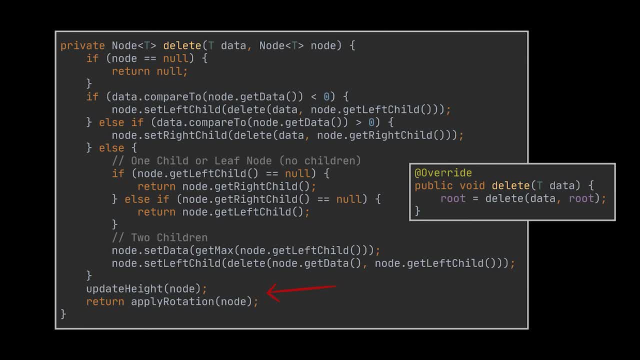 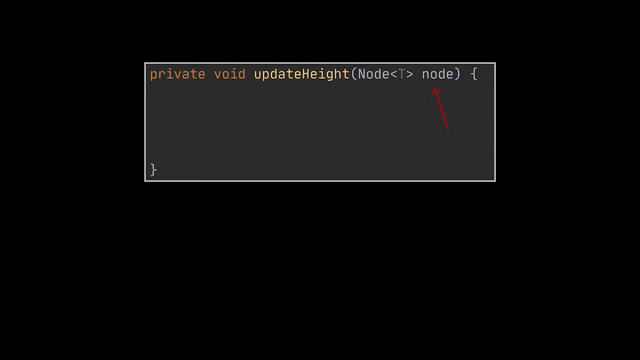 and that our tree is always balanced. Now let's implement the updateHeight and apply rotation methods. Concerning the updateHeight method, this one takes a node as a parameter, because it is the height of this node that we have to update. 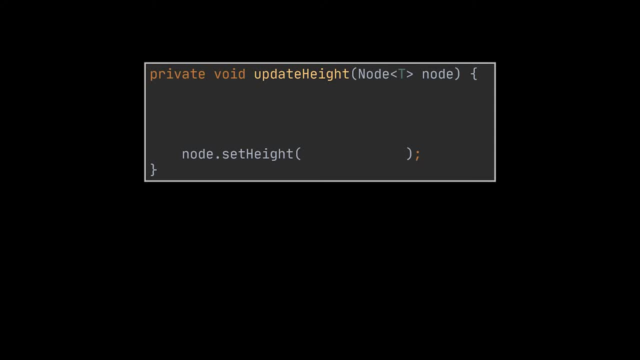 But how are we going to calculate this height? Well, this height is calculated using the height of the children of this node. So we have to fetch the maximum between the height of its left child and right child. Then, because this node is the parent of the node, having the maximum height we just retrieved, 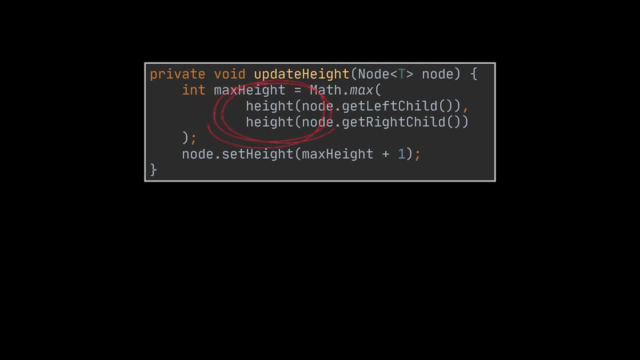 we add one to it. Notice here that I did not retrieve the height of each child using directly the getterGetHeight method. That is because this method might be called on non-existent, But it is not. It is called on null nodes and using the getHeight in such cases will throw a null pointer exception. 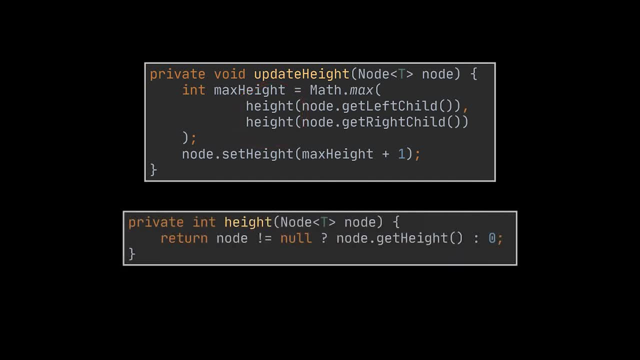 So what we have to do instead is use this helper method, which will check: if the node is different than null, then it will return the node's height for us, And if the node is equal to null, it will return a zero for us. 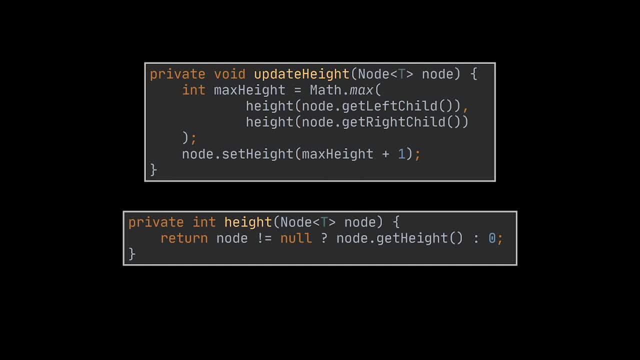 which is the height of every null node in an AVL tree, as we previously mentioned. That is basically all we need to do for this method. Let's go ahead now and implement the applyRotation method, Guessing which of the four cases we need to tackle. 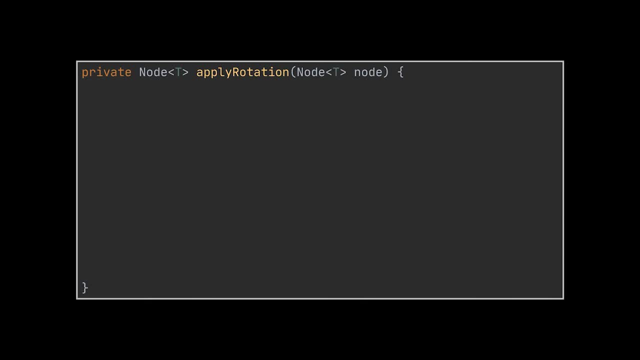 is based on the balance of the node that is being passed to the applyRotation method. So what we have to do first is calculate this balance, and this was done using another helper method. This method will also check if the node we are dealing with is a null node or not. 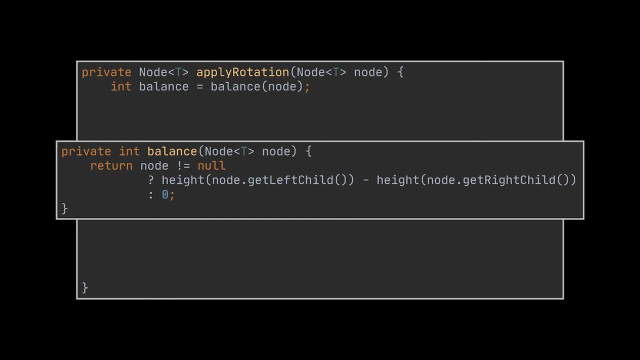 because if it is, we will return a zero. However, if it isn't, we will return the result of the equation we talked about, and it is the height of the left node or subtree minus the height of the right node or right subtree. 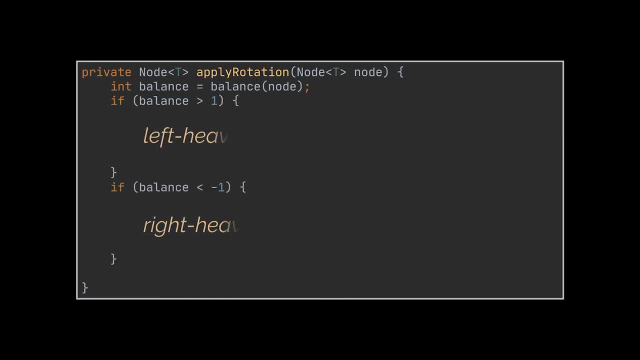 Now that we have the balance, we can check in the applyRotation method if this balance is bigger than one or smaller than minus one. If it is bigger than one, we know we are in a left-heavy situation, and if it is smaller than minus one, 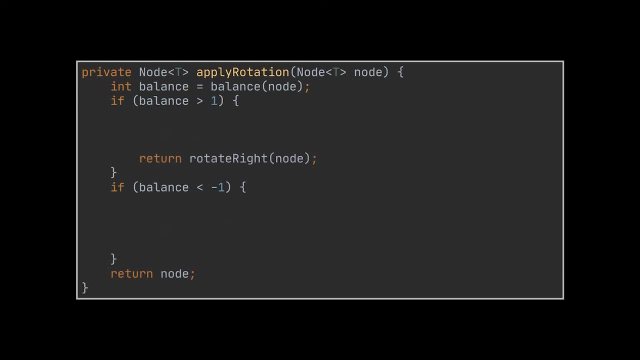 we know we are in a right-heavy situation. So for the left-left situation, we need to apply a right rotation on the node passed to the method, and for the right-right situation, we need to apply a left rotation on this node. However, two cases remain. 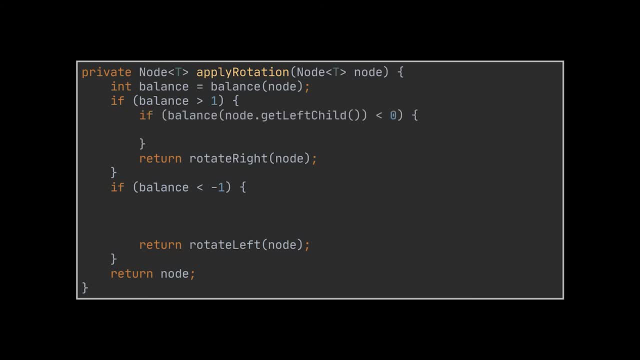 For the third case, we said that if the balance of the node passed to the method is positive and the balance of its left child is negative, then we have to perform a left rotation on its left child, followed by a right rotation on the node itself. 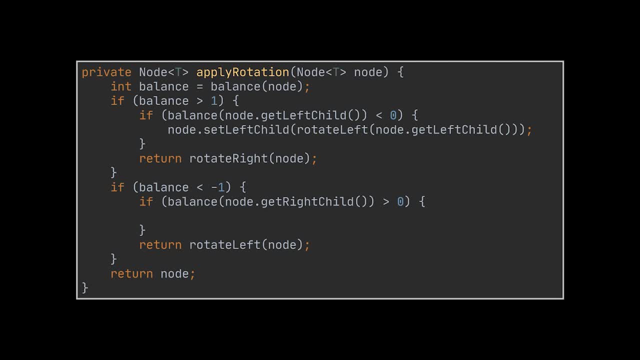 Similarly for the fourth case, we mentioned that if the balance of the subtree's node is negative but the balance of its right child is positive, then we need to perform a right rotation on the right child, followed by a left one on the given node. 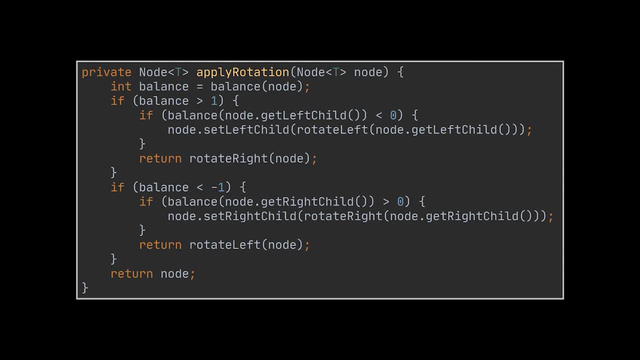 And these if statements are here to do that and ensure that all four situations are covered. Notice also how we are setting the left child and right child of this node respectively and how the nodes are being returned. But why are we doing that? Well, to understand this, 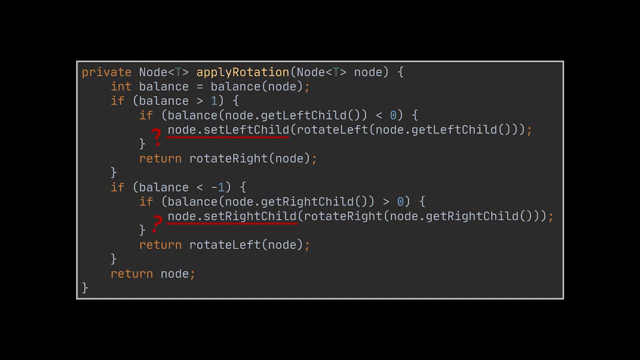 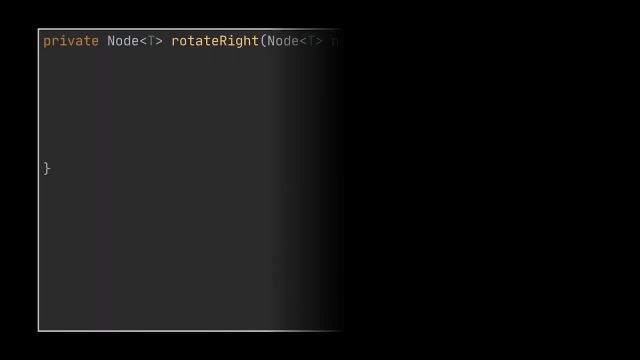 we will need to dive deeper in rotations and follow their mechanism step by step, while implementing the rotate left and rotate right methods. Consider this tree as the tree we need to rotate to the right on node 10,, as the result of this rotation can be seen next to it, to the right. 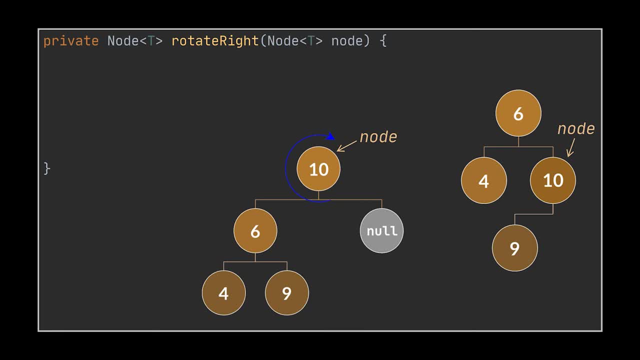 Let's try now to implement the rotate right method. The first thing we need to do is store two nodes inside variables to keep their references. The first one is the left node of the root, or the unbalanced node, and the second one is its right child. 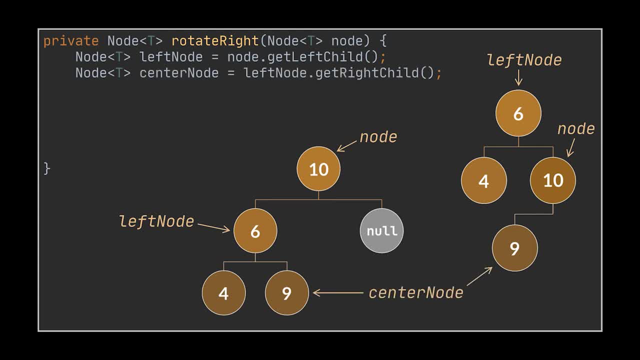 In a left heavy situation. this latter node is equal to null. However, the use case you can see is used to represent the most generic scenario, and that is why we need both of them. Now notice how, after the rotation is applied, 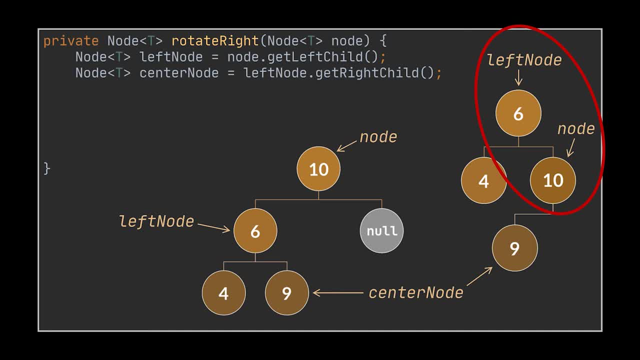 our root node. here the node variable becomes the right child of the left node. So let's go ahead and set the right child of the left node to be the node variable passed to the method. The next thing you can see is that the center node is now the left child. 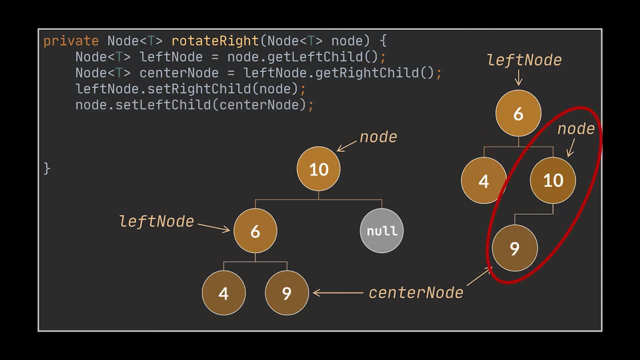 and the right child is now the left child of the left node. So let's go ahead and set the right child of the left node to be the node variable passed to the method. The next thing you can see is that the center node is now the left child of our root node. 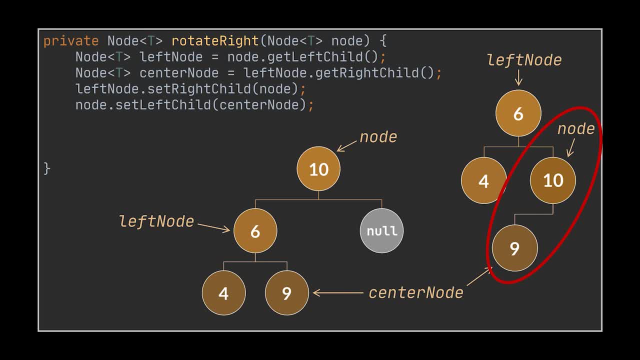 So in code this is also mirrored by setting the left child of the node variable to be the center node. Now, after the rotation is done, the last thing we need to do is update the height of the nodes we moved around. In our case, the height of our root node and its previous left node have changed. 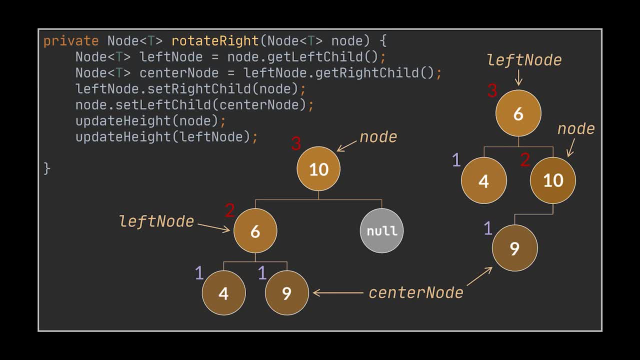 and therefore need to be updated accordingly. This is done using the update height method we previously implemented. Finally, what we need to do is return the node that took the place of our root node. In this example, the left node is now placed in the same position. 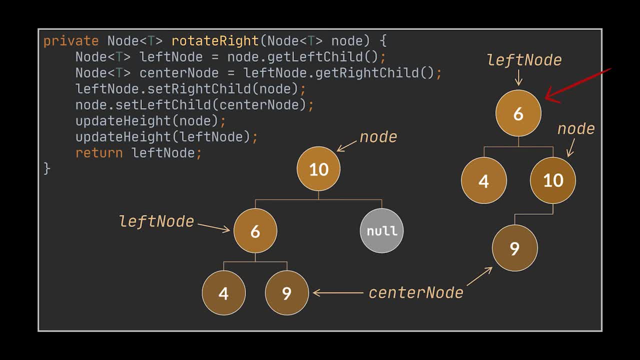 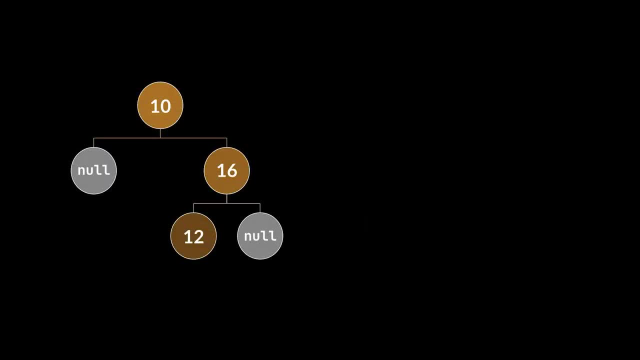 where our root was before the rotation, and hence is the node that should be returned. Now imagine we are in a left-right situation and we have the tree. you can see in front of you When we first apply a right rotation on the right child. 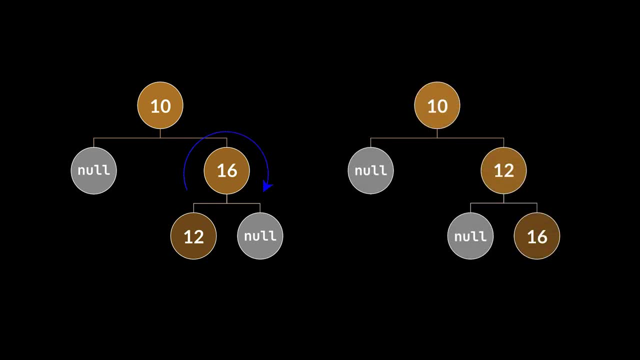 the tree should become something like that: Notice how the right child and its child were flipped. and it is node 12 that is returned by the rotateRight method we just implemented. Now we need something to tell our tree that the child of our root node. 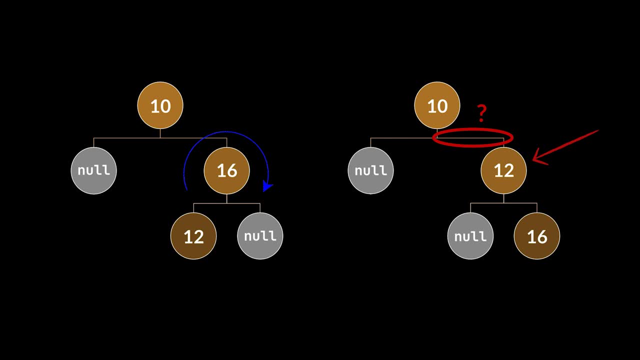 10, has changed and it is no longer the node 16 it used to be. You see, there is no mention inside the rotateRight method to set the child of 10 to be 12.. That is where the setters we added inside the if statements. 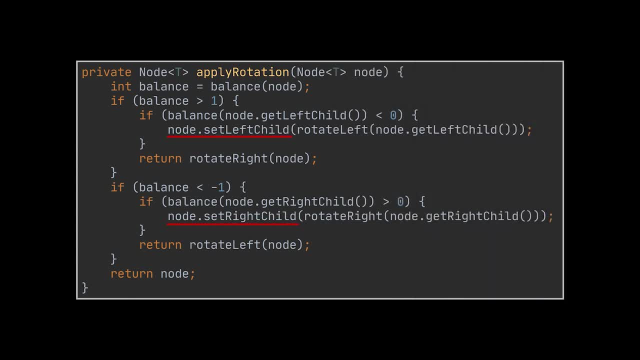 in the applyRotation method come into play, These setters will update the child of the root and put us in an appropriate right-heavy or left-heavy situation respectively, And if you scale things up, the new root returned by the rotate method will also be set as the new child of 10.. 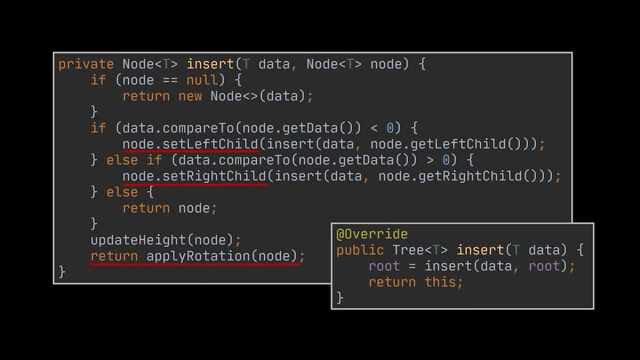 The new child of its parent if it has one. because of the recursive insert calls and the insert method we saw a few minutes ago and implemented in the last video. Now, concerning the rotateLeft method, it should be pretty easy by now. 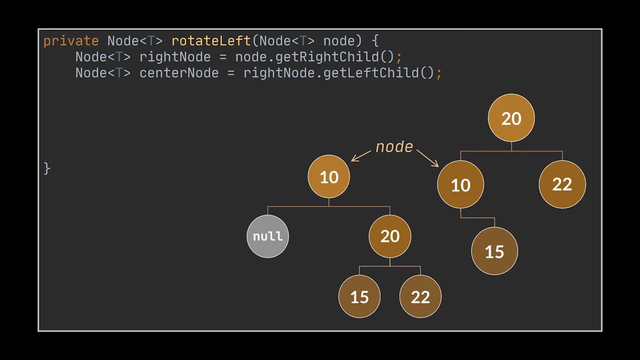 as it is the symmetric case to the one we just implemented. Similarly to what we did with the rotateRight method, we have to start by storing a reference to the right node and the center node, Then we have to set the left child of the right node to be the root.